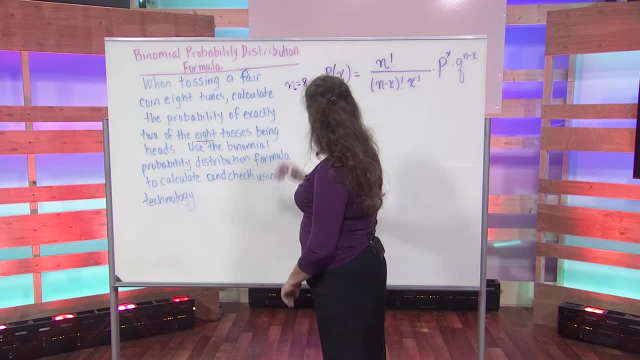 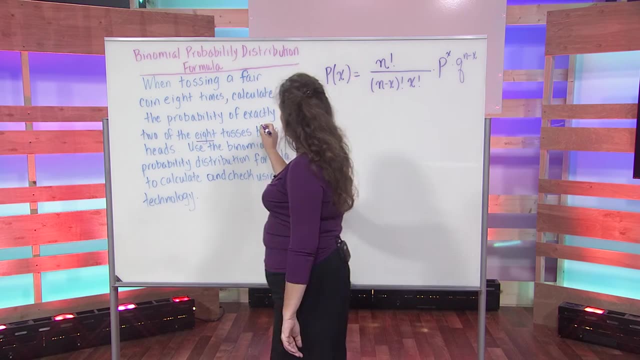 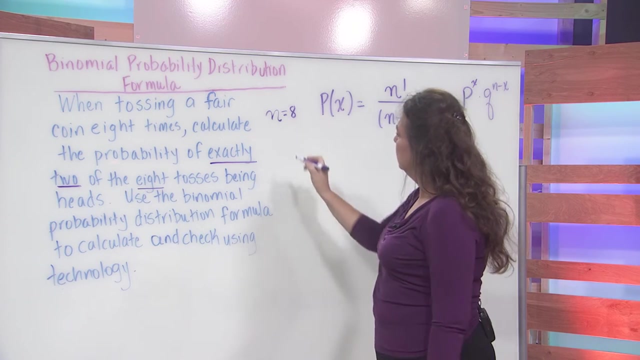 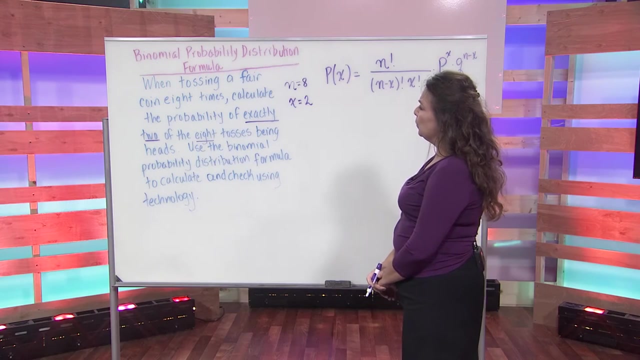 here N is equal to eight. We want to find the probability that X is exactly equal to two. So this: exactly two of the eight tosses are heads. So that is our X is equal to two. Now, it's a fair coin. We're told that in our problem. 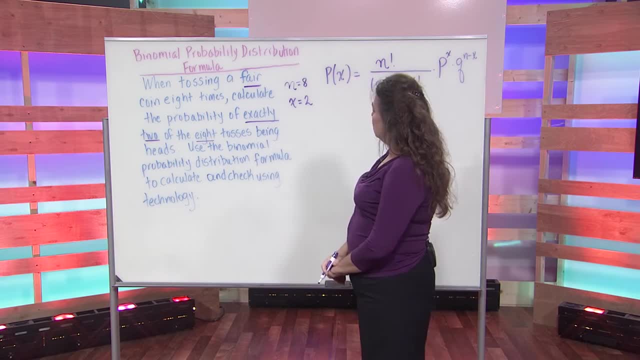 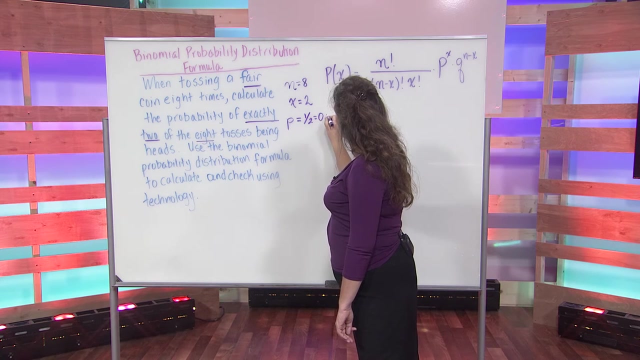 that we have a fair coin. So the probability of getting a heads- we'll write that as P, the probability of a success. in this case, the probability of getting heads on this fair coin is one out of two. one out of two, Or, if I wrote that in decimal format, that's equivalent to: 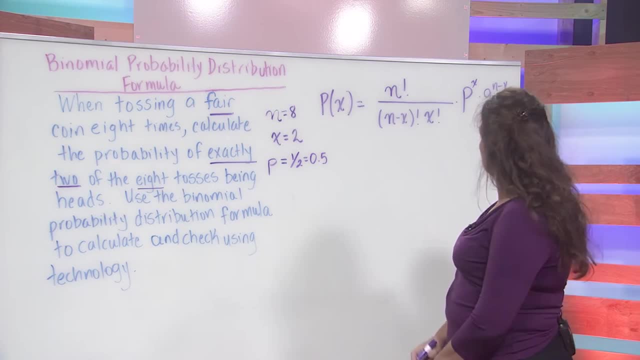 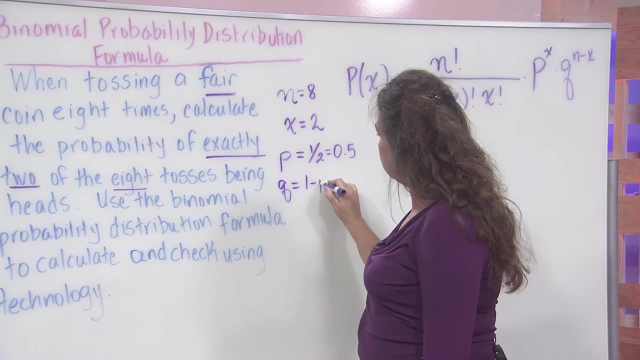 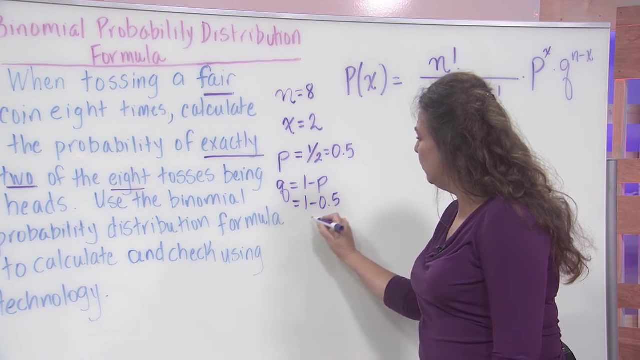 0.5.. Now to find Q, which is listed in our formula. here we'll take Q is equal to one minus P, So we have an idea of what P is 0.5.. So then Q is one minus 0.5 or 0.5 as well. So the probability. 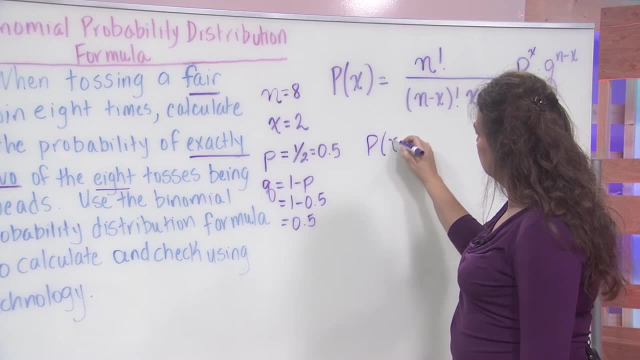 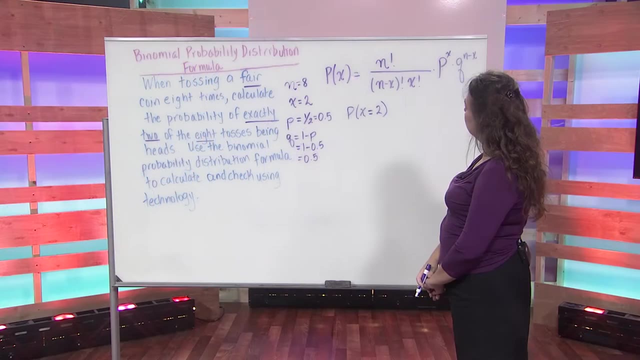 that we want to calculate is the probability that X is equal to two. And from here we want to go ahead and input our information into our formula and go ahead and work out that math. In the numerator we have eight factorial. in the denominator we have eight minus. 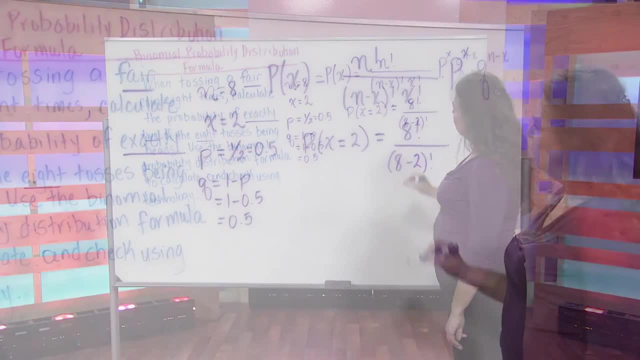 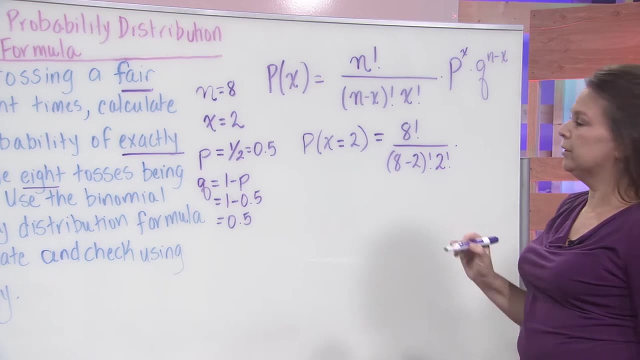 our X and our X is two, two factorial over our X, which is two factorial times our P, which is 0.5, 0.5 to the X, the power of X, power of X plus, which is 0.5, which is 0.5 to the X, the power of X. 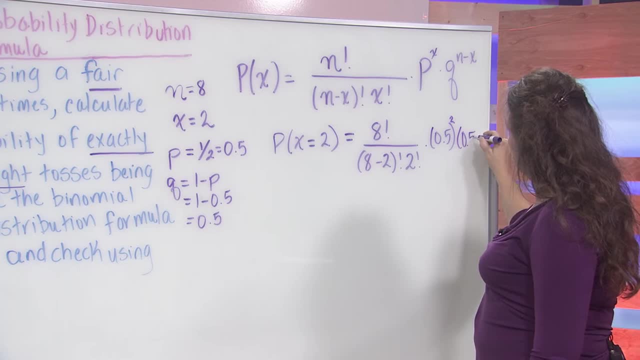 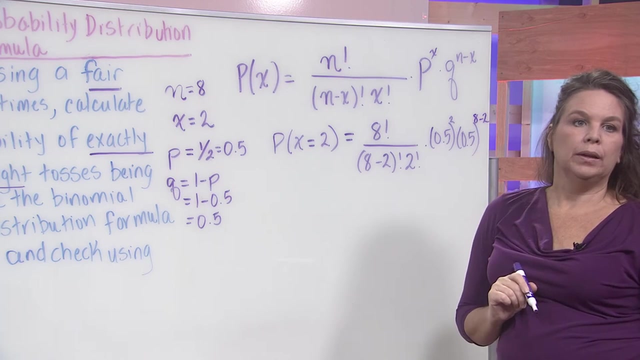 and our X is 2 times 0.5. and then here for the Q we have that to the power of n minus X. so our n we have listed as 8, 8 minus 2, and from here we'll start to work through the arithmetic. so for the time being I'm going to leave that. 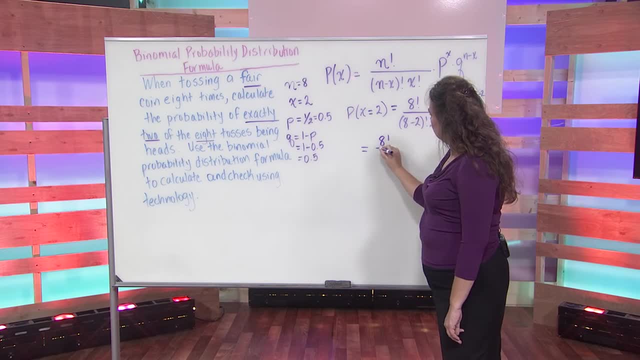 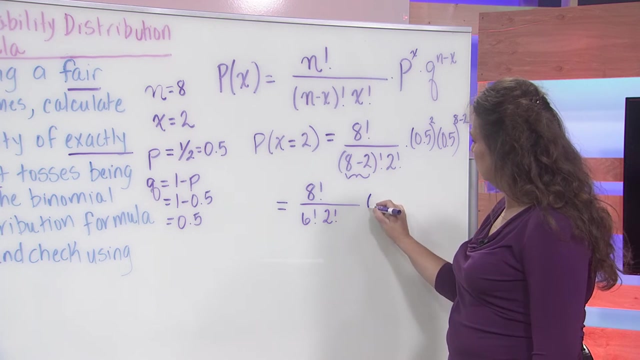 numerator alone. I'm going to write that as 8 factorial and I'm going to simplify a little bit here in the denominator. so we have 8 minus 2. 8 minus 2 is 6 factorial and also bring that down, that 2 factorial, and then here we have 0.5. 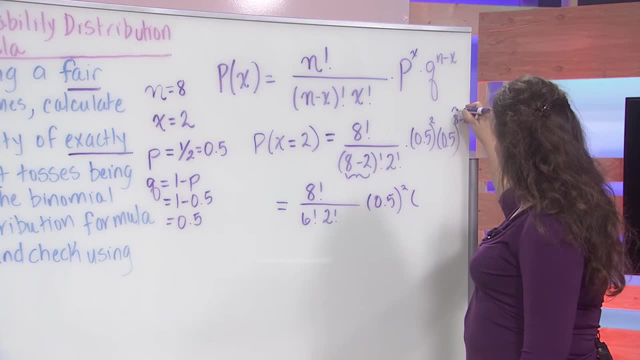 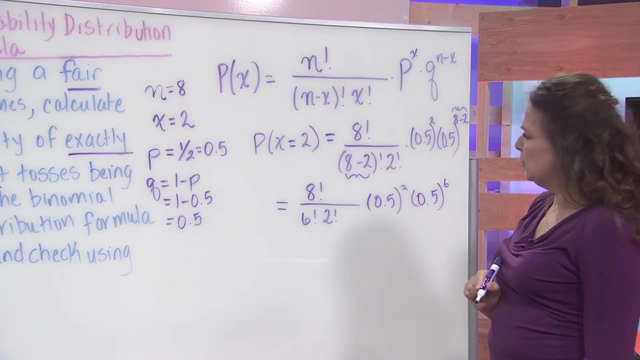 raised to the second power, and I'll go ahead and simplify this: 8 minus 2 as well. so we have point 5 raised to the 8 minus 2, where that gives us 6 to the 6 power. okay, Now I want to think about this expression for a minute. 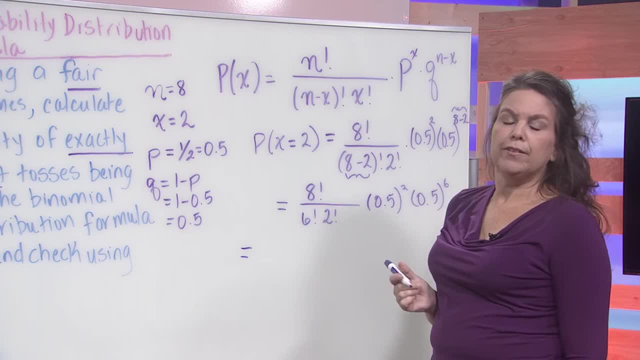 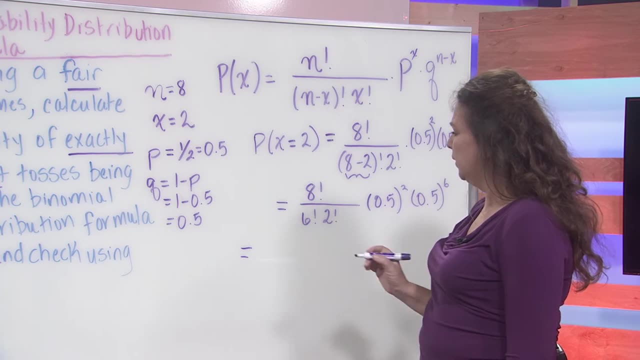 So we have 8 factorial. 8 factorial is 8 multiplied by 7 times 6 times 5, all the way down to 1.. So the way I'm going to write that- and I can simplify that nicely- is 8 times 7,. 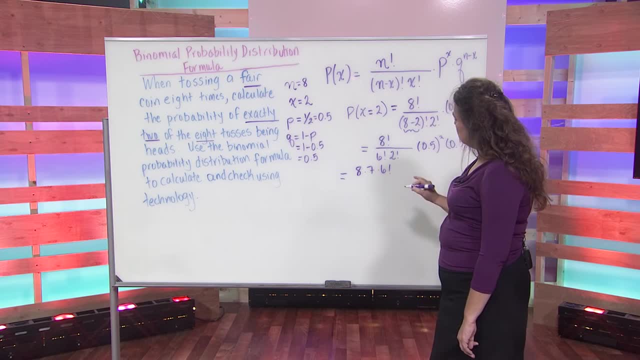 and I'm going to stop at 6. 6 factorial. and the reason I'm stopping at 6 is because I have a 6 factorial here in the denominator. So if I have a 6 factorial in the numerator and a 6 factorial in the denominator, 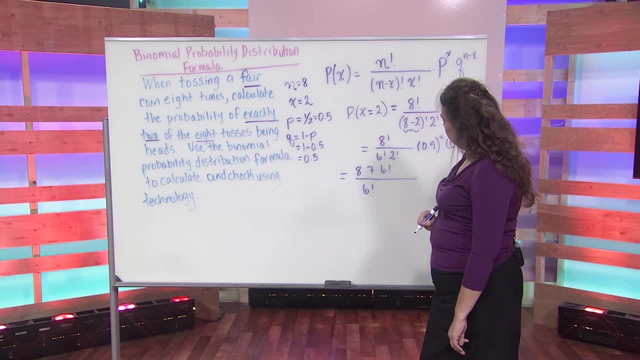 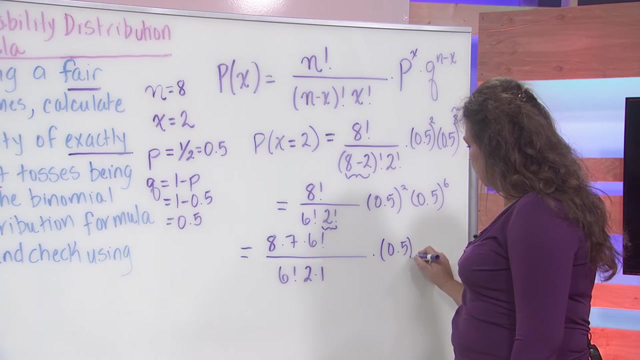 those will divide one another out. So we have 6 factorial in the numerator, 6 factorial in the denominator, and then this 2 factorial here. Well, that's equivalent to 2 times 1. And I'll go ahead and bring along the 0.5 raised to the second power. 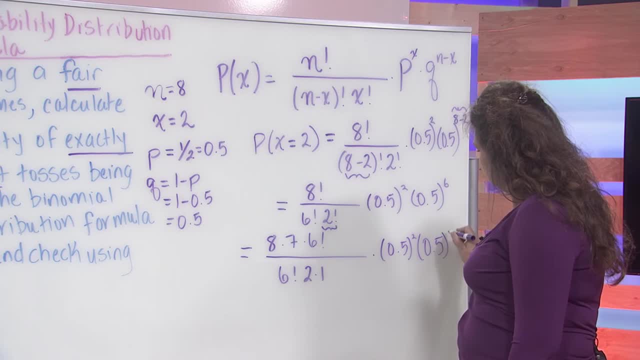 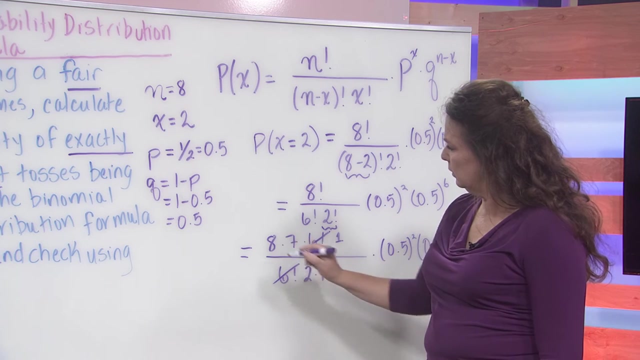 and the 0.5 raised to the sixth power. So these numbers are the same. They divide out to 1.. And then what we're left with in the denominator is 2 times 1.. Well, 2 goes into 8 evenly. so we can simplify here as well. 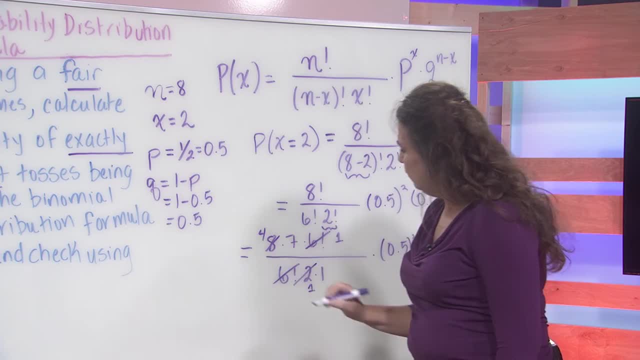 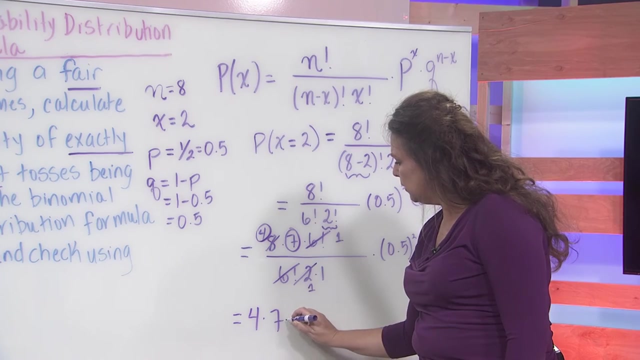 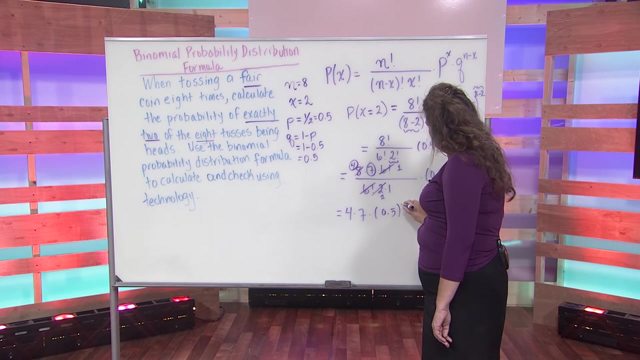 2 goes into 2 once, 2 goes into 8 four times. So now what we're left with, regarding this expression involving factorials, is the 4 times the 7 times the 1.. Okay, So we have 4 times 7, and then the 0.5 raised to the second power. 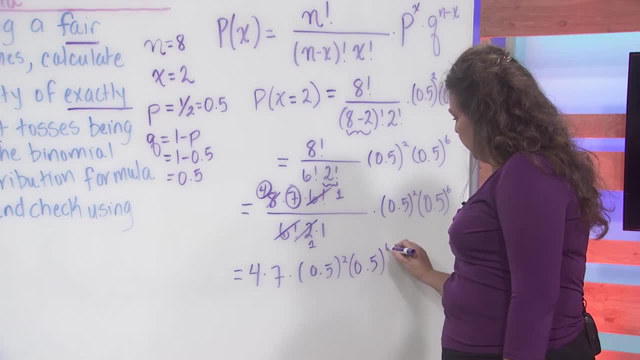 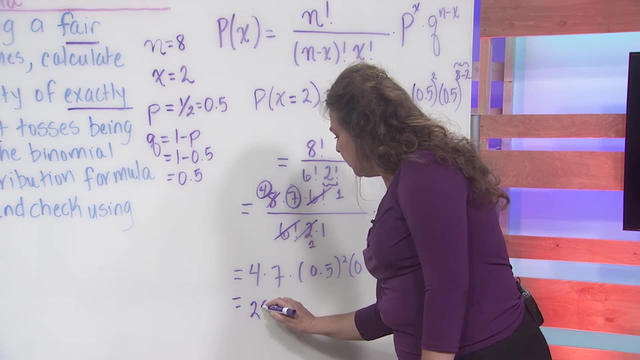 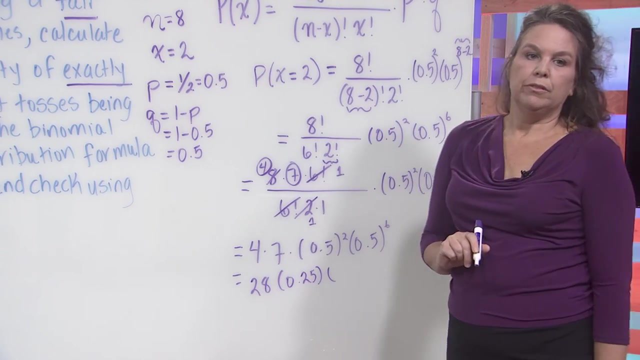 and the 0.5 raised to the sixth power. So now we want to plug this into our calculator. If we do that, we get 28 here. This is going to give us 0.25 here, 0.5 raised to the sixth power.